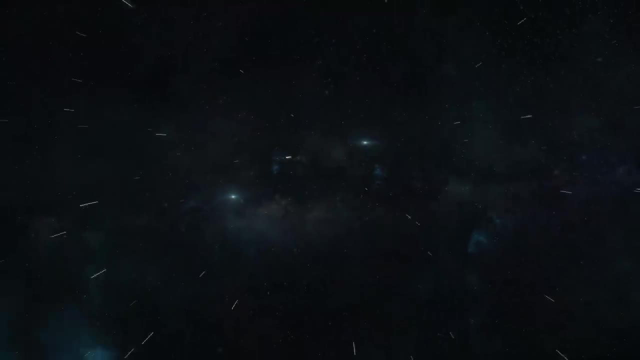 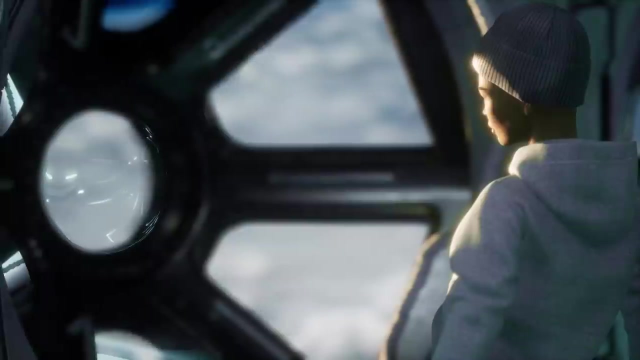 The vast distances between stars and the large number of threats lurking in outer space make interstellar travel difficult and potentially dangerous. If we're being honorable about the risks that many places have to face and the risks that we may encounter, we can have a tough time understanding them, But we're also 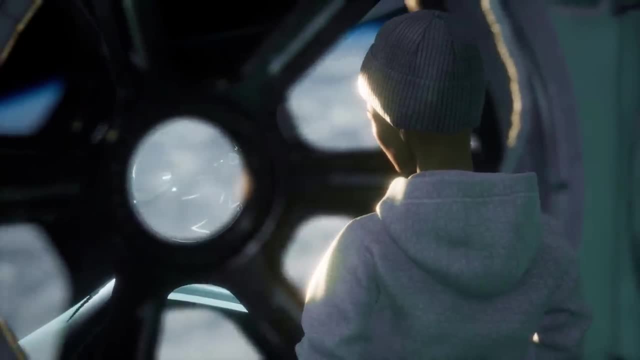 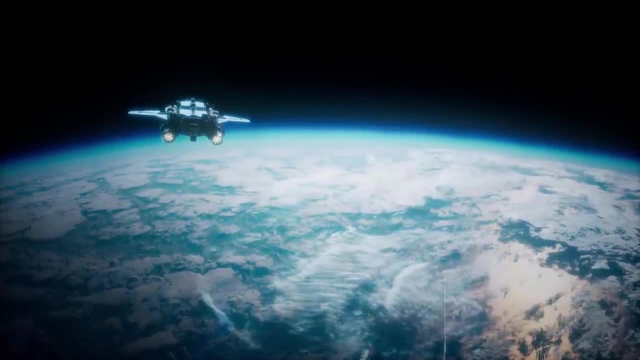 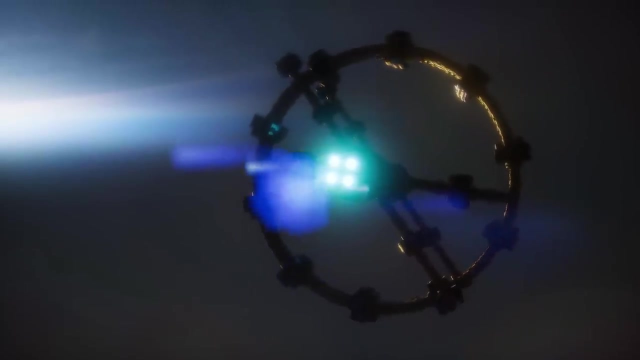 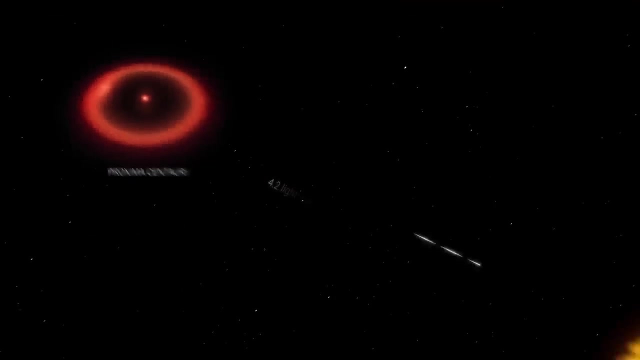 optimistic and certainly not unrealistic: humans will be able to achieve interstellar travel within our lifetime. The possibilities are endless and the rewards could be extraordinary. The difficult task of interstellar travel is primarily defined by the vast expanses between stars. Our closest neighbor, Proxima Centauri, is a little over 4.2 light-years away. This means 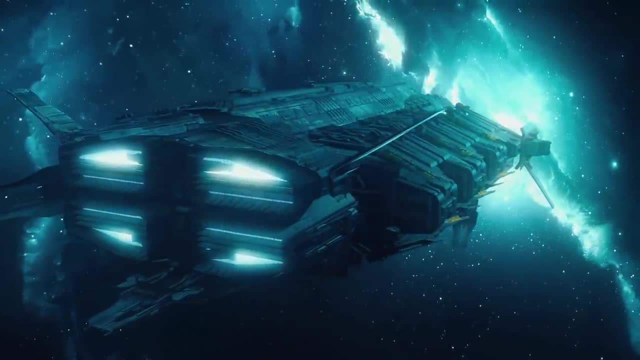 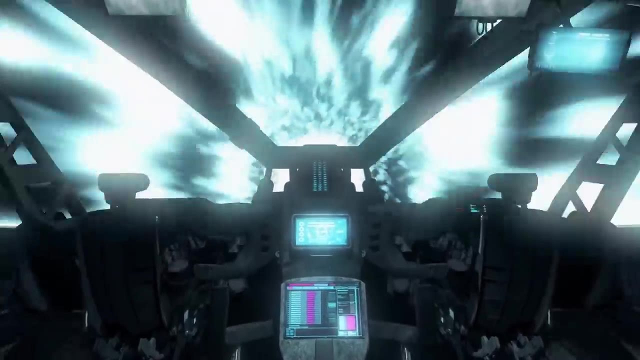 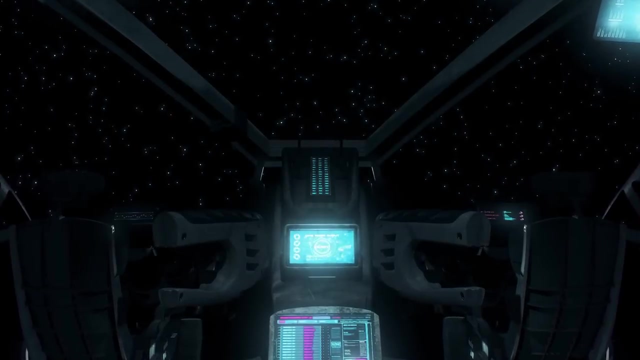 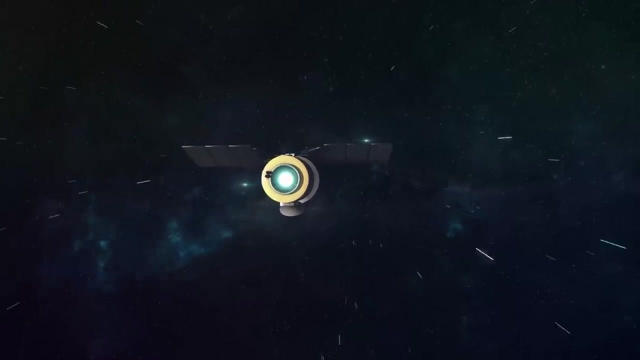 that even if we traveled at the maximum speed currently possible in the universe, which is the speed of light, the journey would take more than four years. Despite contemporary advancements in technology, achieving these speeds is still impossible. Even with the most advanced propulsion technology currently available, such as nuclear or ion propulsion, it would take a 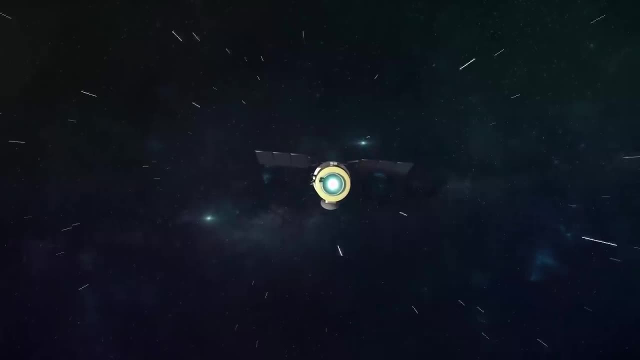 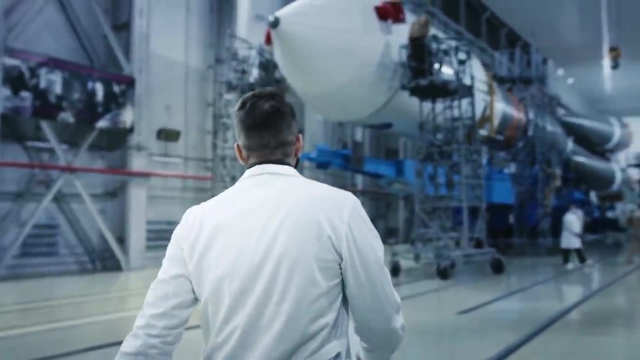 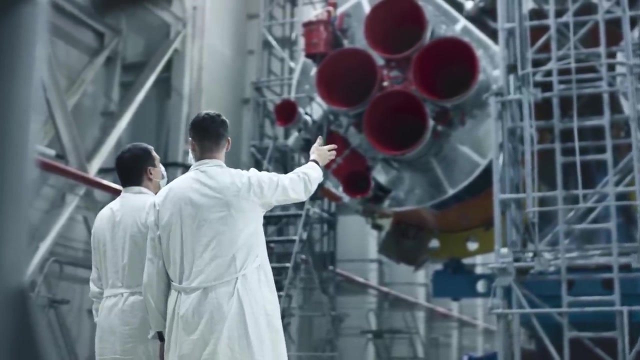 spacecraft decades, if not centuries, to reach the nearest stars. To overcome this problem, the best option is to develop new engine technologies that can achieve much greater speeds. Various concepts on how to achieve that are being considered, including the idea of using antimatter, thermonuclear fusion or even harnessing 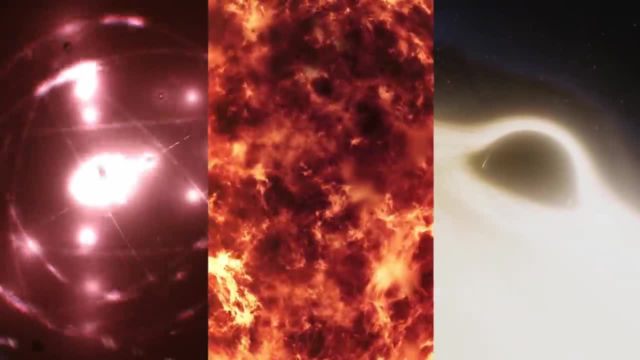 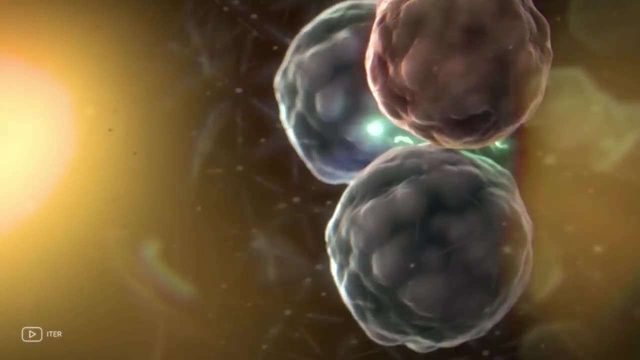 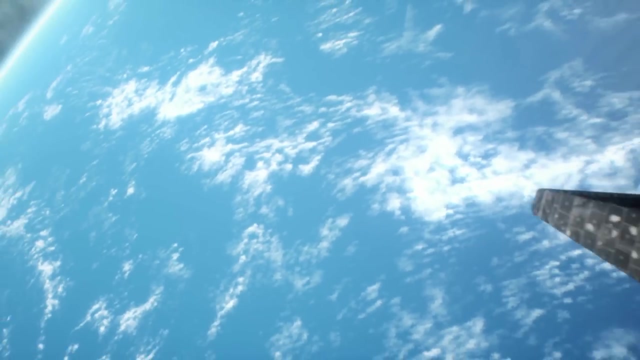 the forces of black holes. Nuclear fusion, the process that powers the sun and other stars, involves combining two light atomic nuclei, such as hydrogen, to form a heavier nuclear, which is called the nucleus, and release the energy. Although nuclear fusion technology is 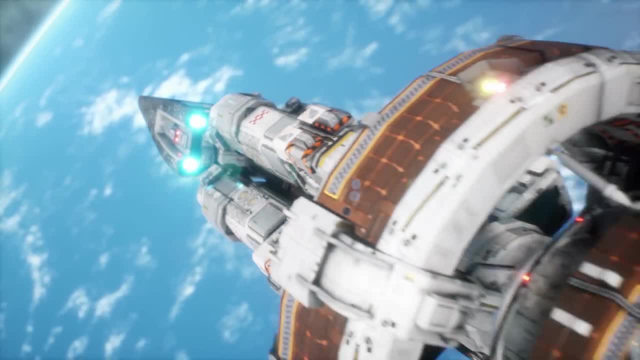 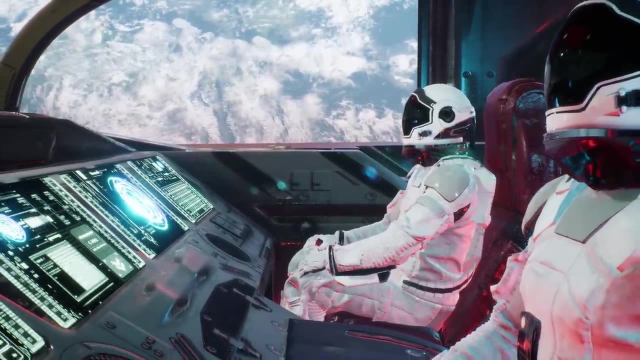 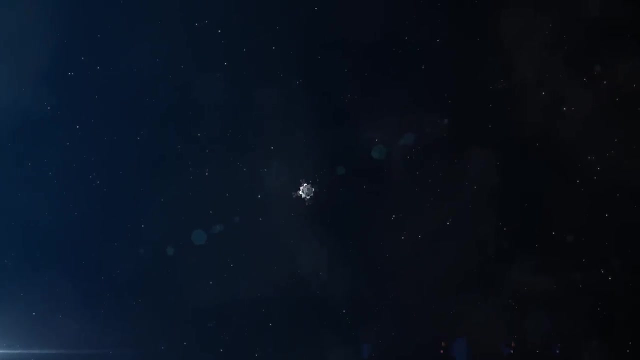 still in its infancy on Earth, it has the potential to provide an almost limitless source of energy and could be used to power spacecraft engines. However, these feats of technology are still purely theoretical and there is no telling whether they will ever be possible in practice. 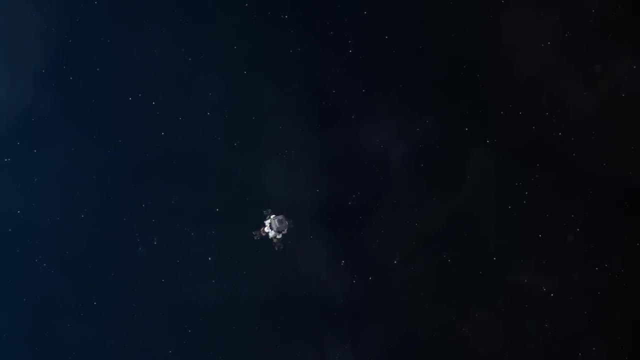 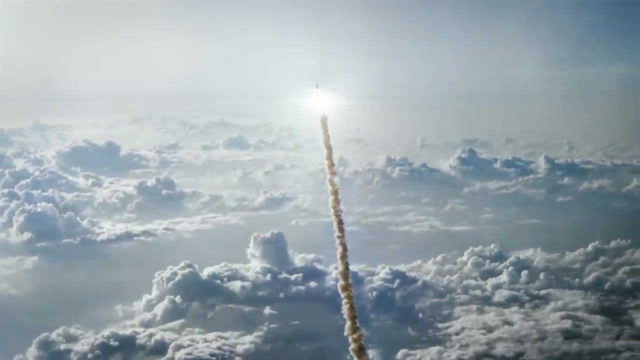 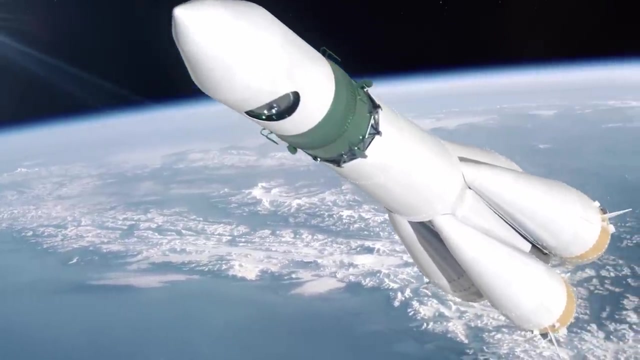 or safe enough to use. The complexity of interstellar travel as a concept is a very important part of our research, and it is exacerbated by the astronomical amount of fuel and energy required to travel such great distances. The traditional rocket propulsion technology relies on huge amounts. 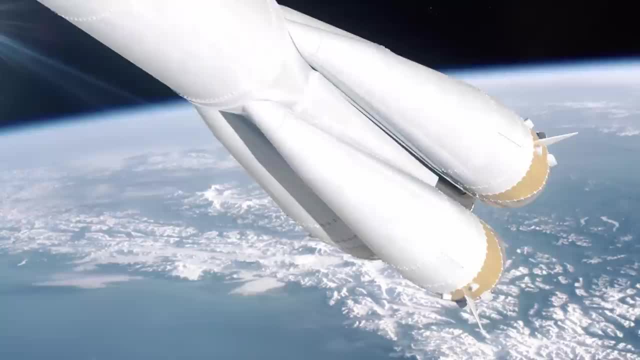 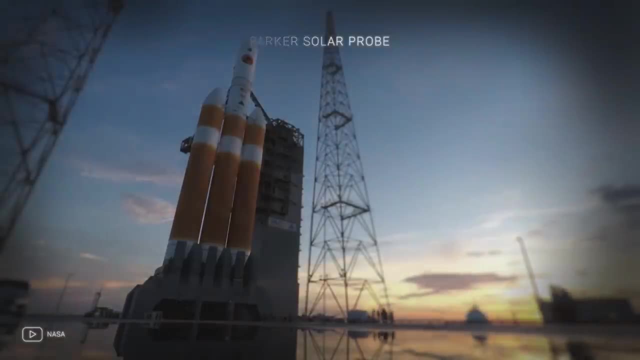 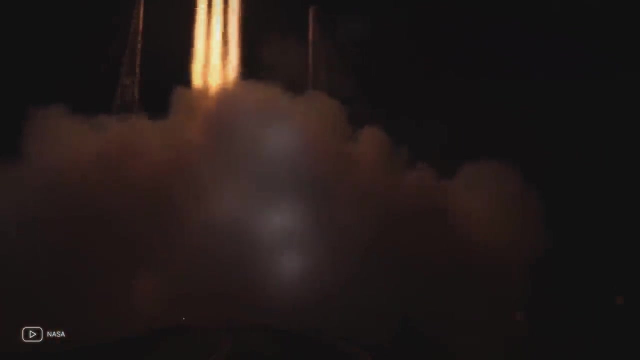 of fuel, propelling spacecraft at a speed only a fraction of the speed of light. For instance, the Parker Solar Probe is the fastest traveling spacecraft ever built by humans and can only reach the speed of 119.4 miles per second. For reference, this is only the 0.064 percent of the speed of light. In order for us to reach Alpha Centauri in human lifetime or less, we need to figure out how to develop a speed of at least 10 percent of the speed of light. However, the 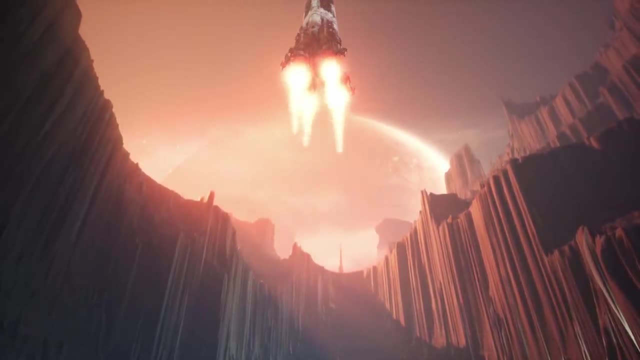 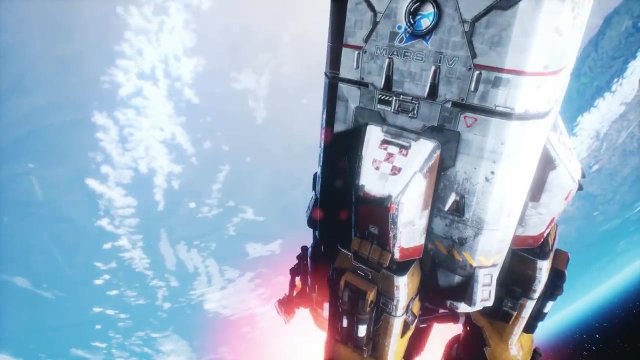 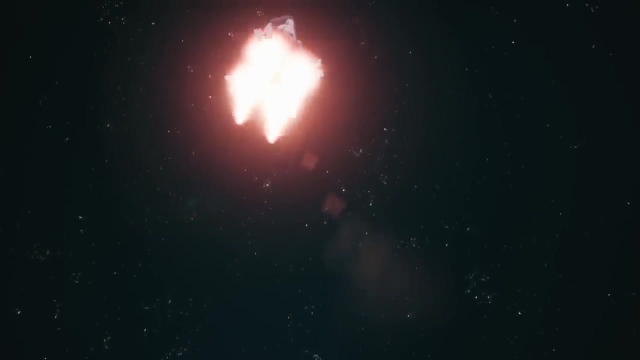 paradoxical nature of this task is that, in order to increase the speed of the spacecraft, we need more fuel. By carrying more fuel on board the ship, the weight of the vessel increases, which subsequently reduces its speed. Sounds like a vicious circle. 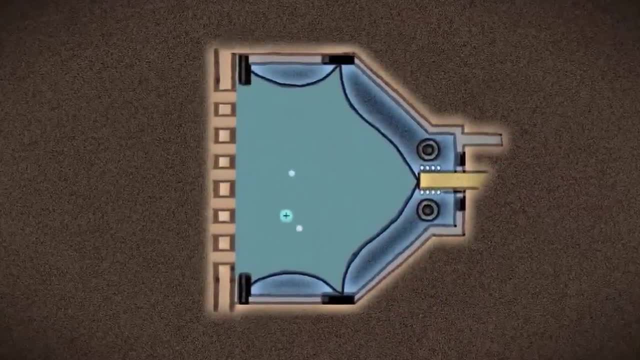 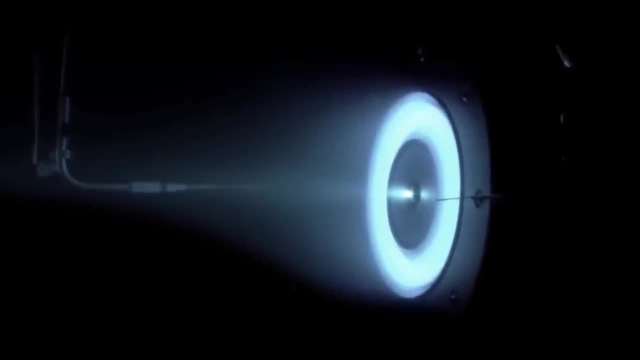 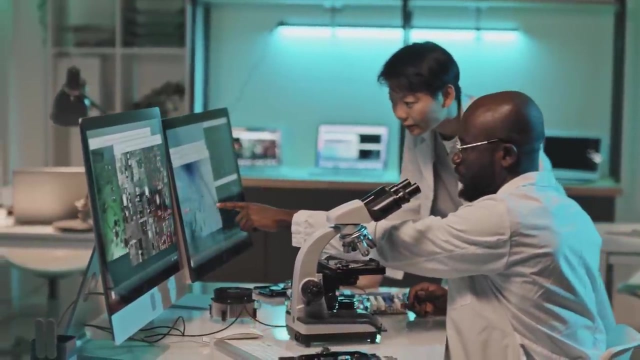 Nuclear or ion propulsion engines are the most advanced propulsion technology that is currently available, Offering much greater efficiency in terms of fuel consumption, they still require a significant amount of fuel to generate the required power. To overcome these obstacles, researchers are developing completely new propulsion technologies that 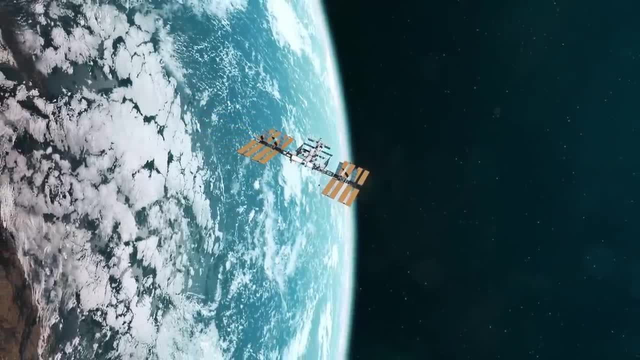 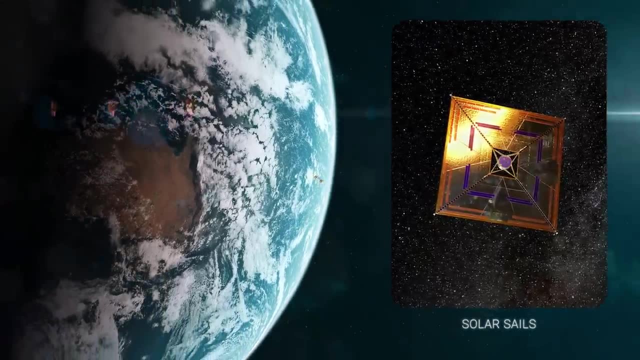 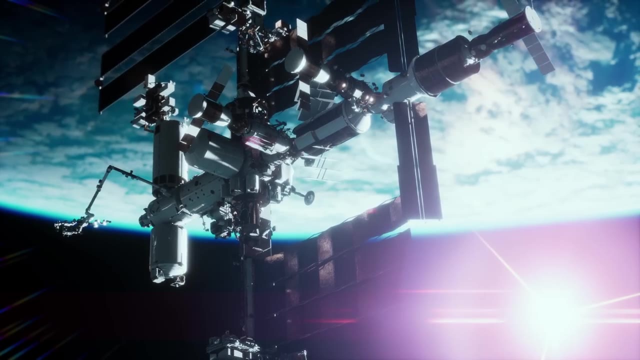 could harness the energy sources available in space. For instance, scientists are exploring the possibility of using solar sails, which use the energy coming from the sun, similar to the way regular sails use the wind, to ensure the continuous acceleration of the spacecraft. Another solution that has been put forward is to use antimatter propulsion, which would 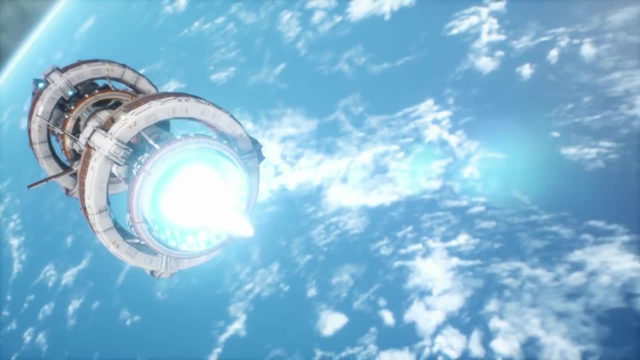 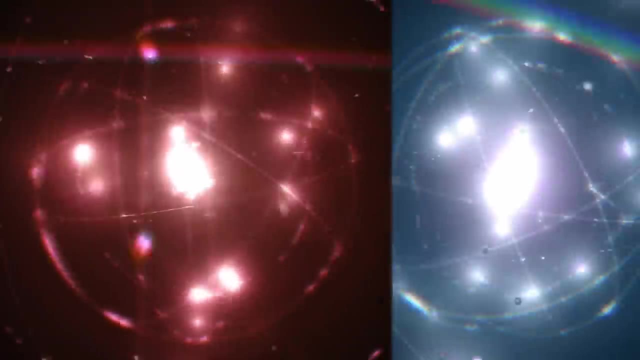 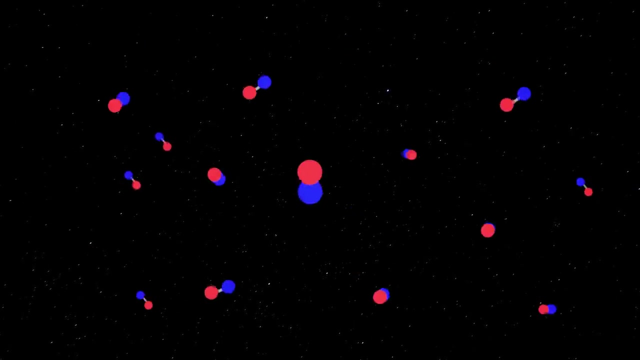 allow the spacecraft to achieve much greater speeds while consuming less fuel. Antimatter is a unique substance that has the same mass as regular matter, but with the opposite electric charge. When matter and antimatter come into contact, they annihilate each other, releasing tremendous amounts of energy. Antimatter is capable of delivering. 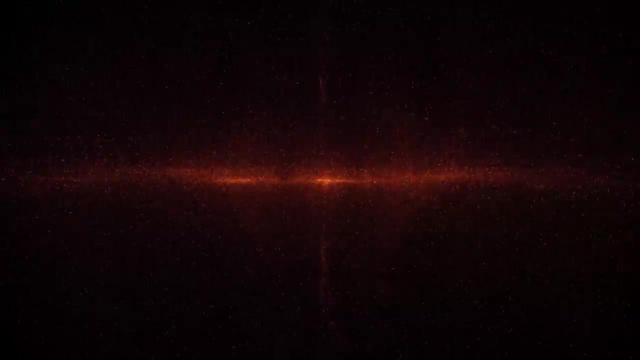 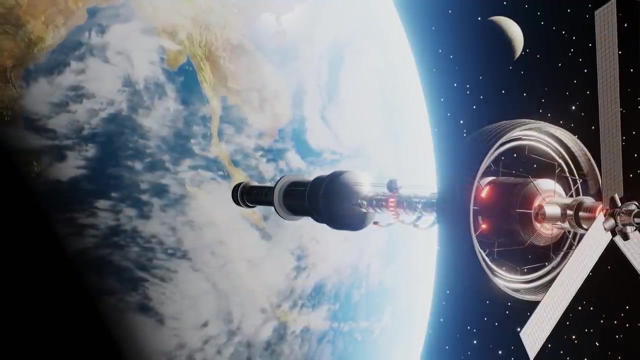 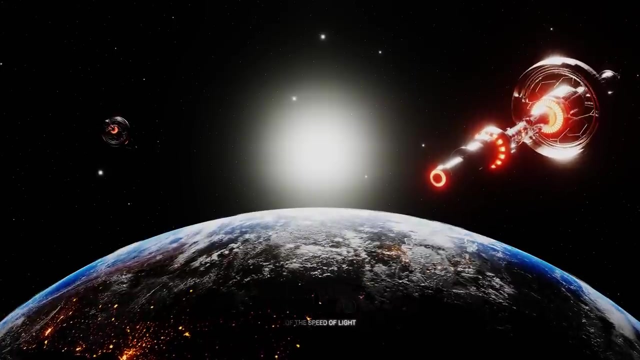 much denser energy than any technology currently available. Theoretical calculations suggest that a spacecraft functioning on antimatter could potentially reach up to 90 percent of the speed of light. This would mean it could reach Proxima Centauri in just over four years. 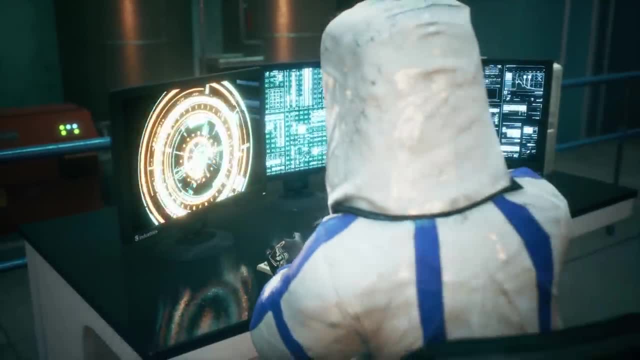 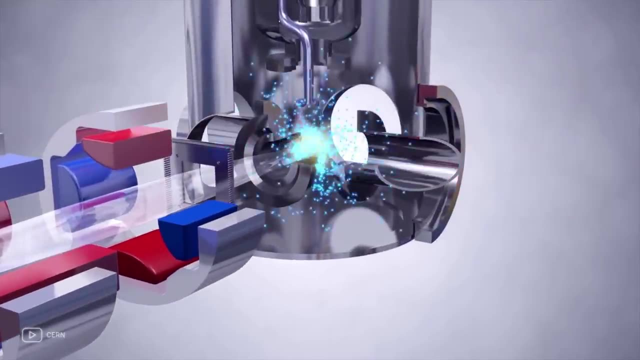 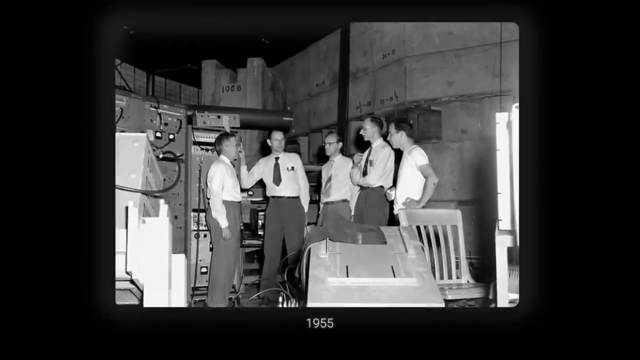 Scientists have been conducting experiments with antimatter for decades. One of the earliest experiments involved creating antiprotons, which are the antimatter equivalent of protona. The first antiprotons were generated in 1955 by a group of scientists at the Lawrence Berkeley. 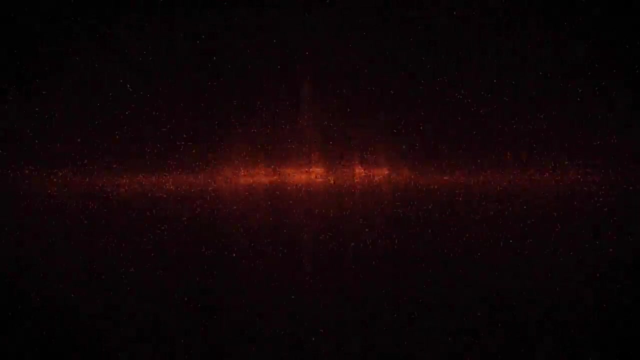 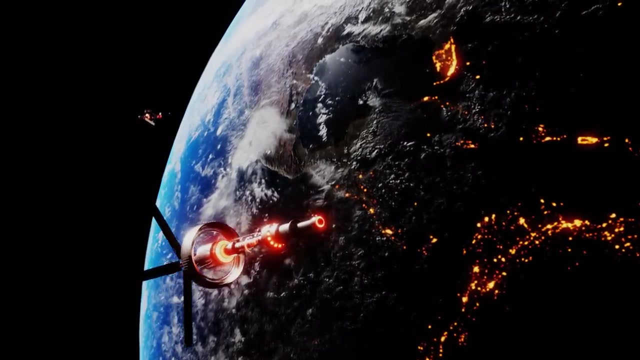 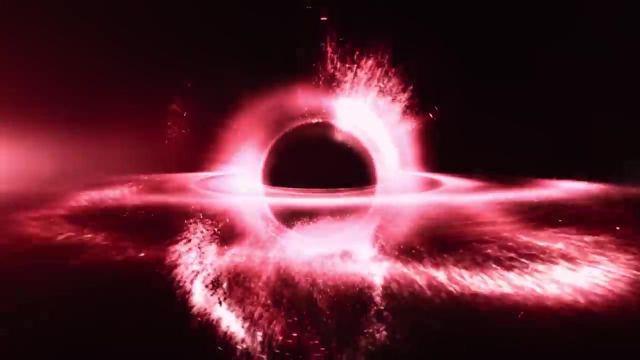 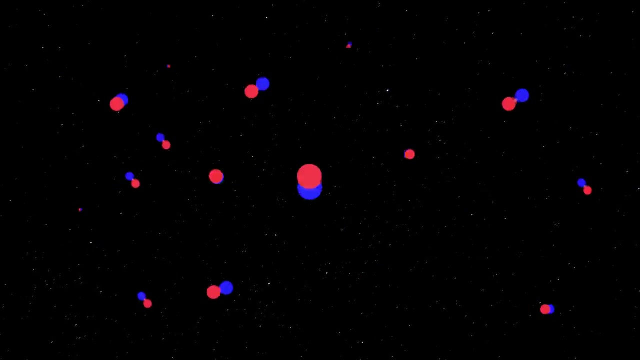 National Laboratory in California. However, antimatter is very costly and difficult. The technology to use it for propulsion is still at an experimental stage. Furthermore, antimatter is highly unstable and difficult to store. Its particles cannot be stored in a traditional container, as they would quickly come into contact with matter and destroy. 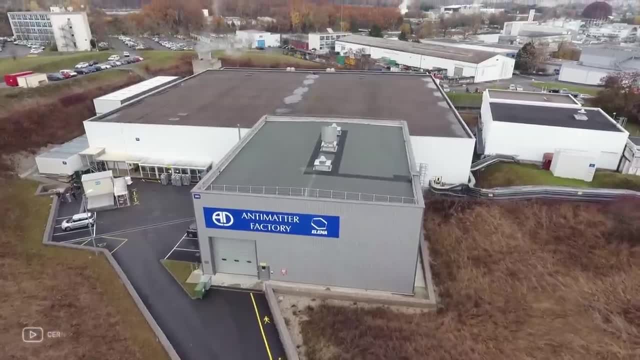 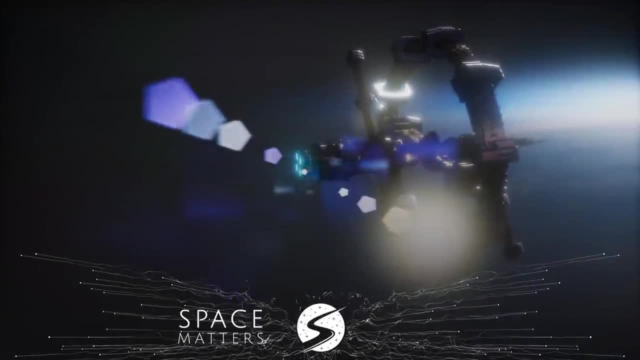 each other. Instead, magnetic fields were developed specifically for the task of capturing and storing antimatter. To sum up: the need for a large amount of antimatter to be stored in a container would be extremely difficult. To sum up: the need for a large amount of antimatter would be extremely difficult. 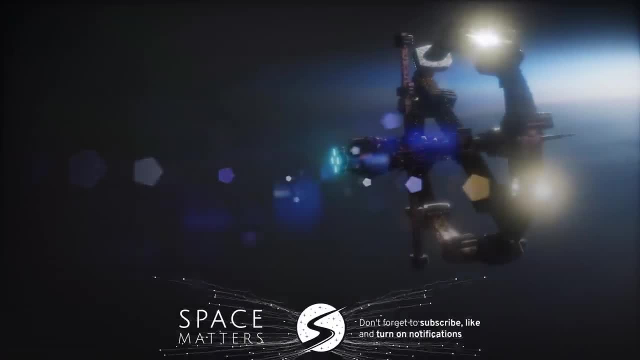 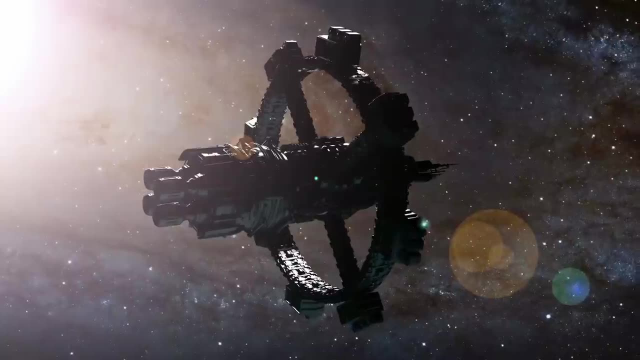 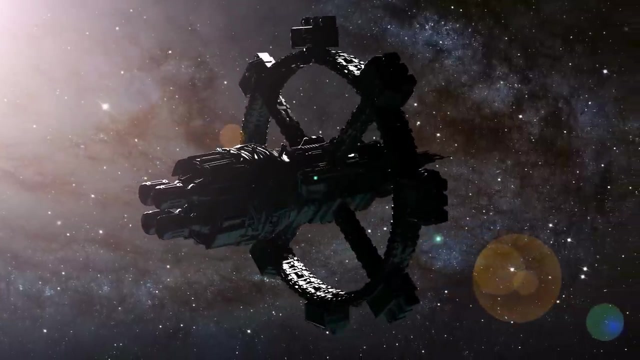 In some cases, large amounts of fuel and energy for interstellar travel poses enormous challenges. However, developing a completely new propulsion technology-or harnessing energy from sources available in space-is definitely a necessary push in the right direction. Once we find a way to travel fast enough, we still won't be ready for interstellar 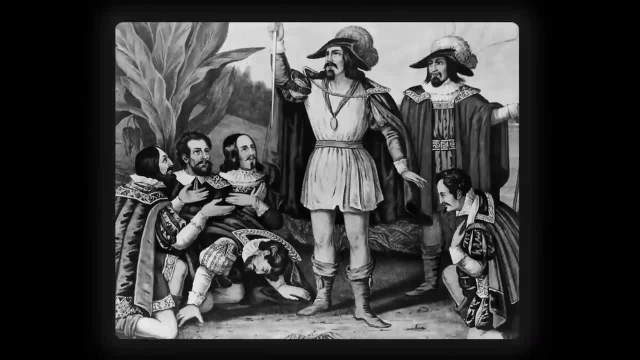 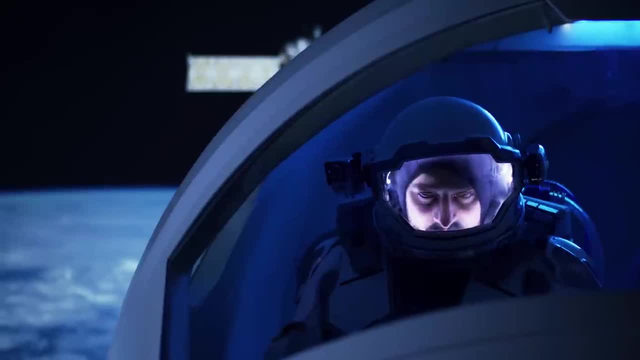 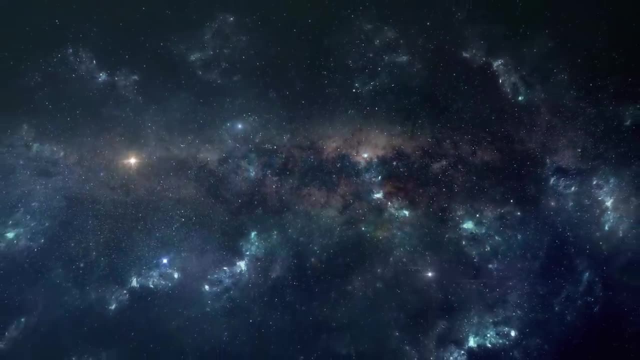 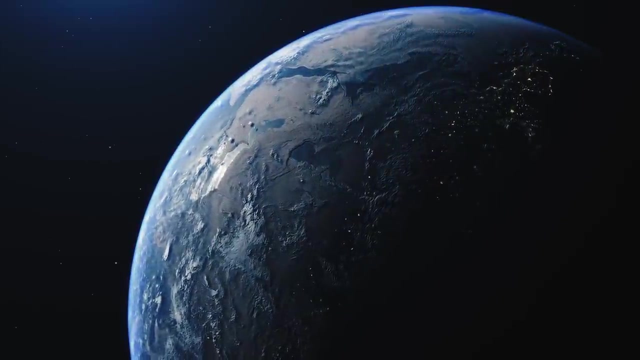 travel, since even Columbus did not travel blindly in his search for a new route to India: to India. Navigation and communication during interstellar travel present another major challenge for manned missions. The great distances between stars means that there could be significant delays in communication with Earth. This would make real-time communication difficult or even 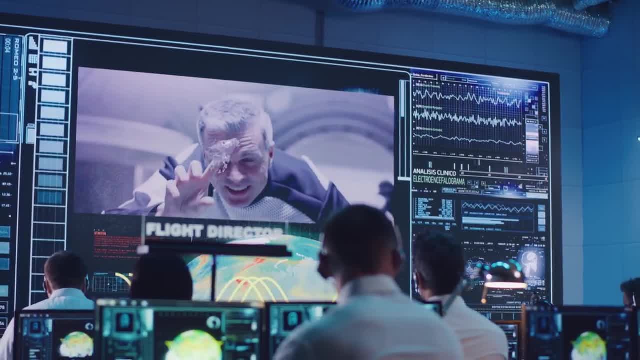 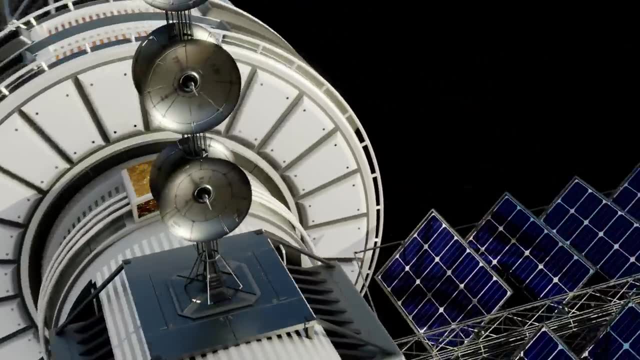 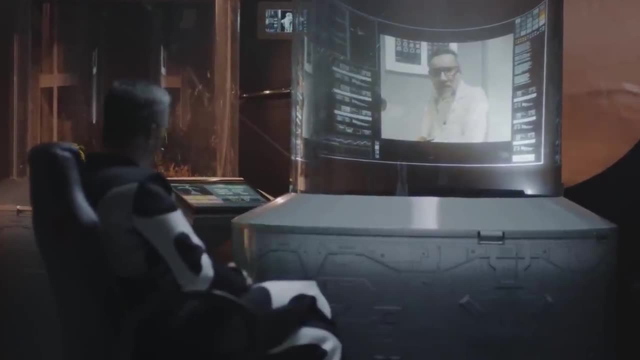 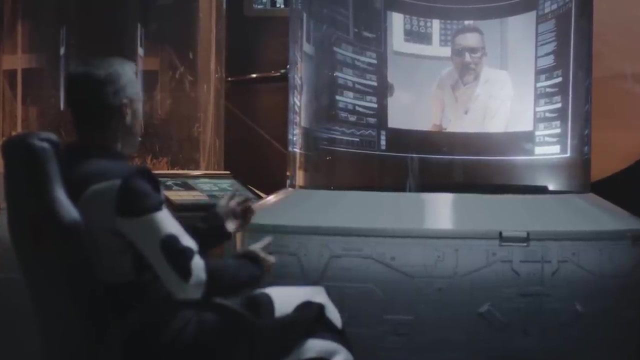 impossible. Furthermore, signals from Earth could be faced with interference noise or they could become completely lost, making data acquisition and interpretation very difficult. To resolve these issues, spacecraft will require advanced communication and navigation systems capable of handling the unique demand of interstellar travel. One possible way to do that is to use 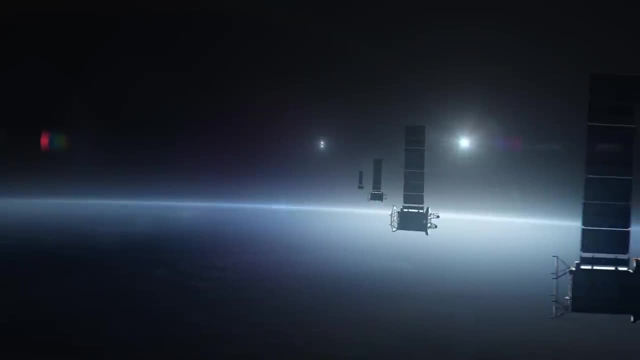 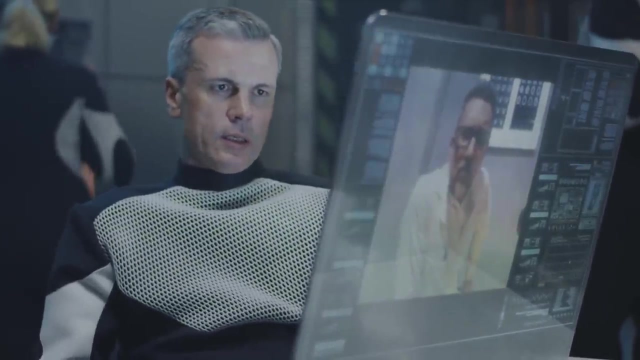 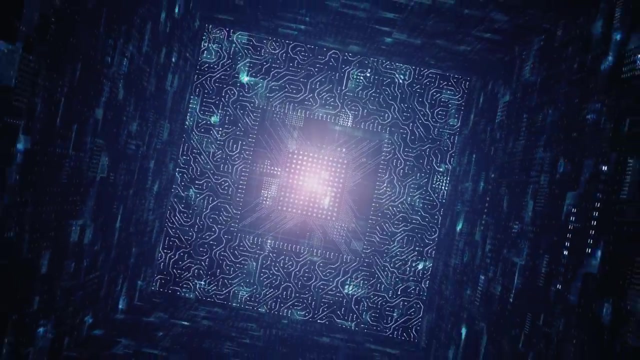 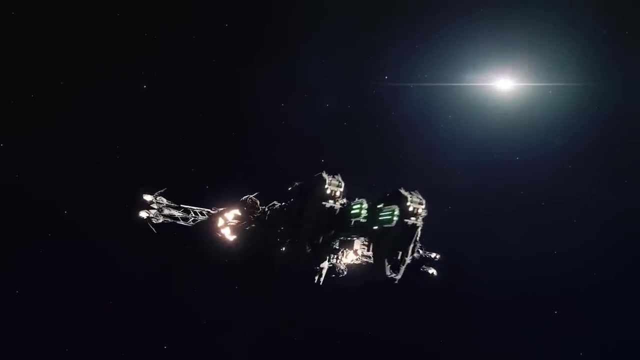 a network of interstellar satellites that could relay information between Earth and the ship, ensuring faster and more reliable communications. Another promising solution is quantum communications technology, which uses entangled quantum particles to transmit information instantaneously over long distances. This technology could revolutionize interstellar communications by allowing real-time transmission. 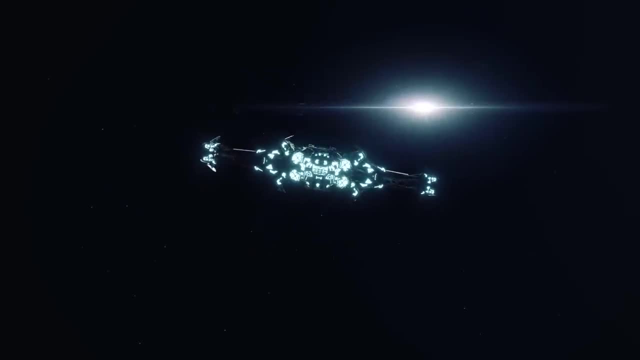 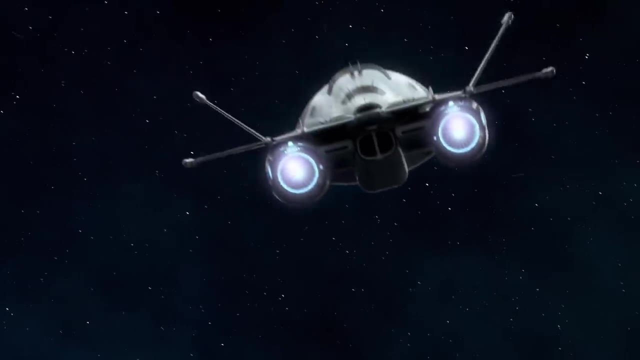 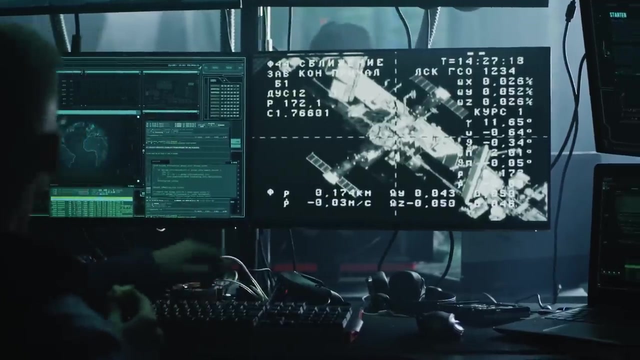 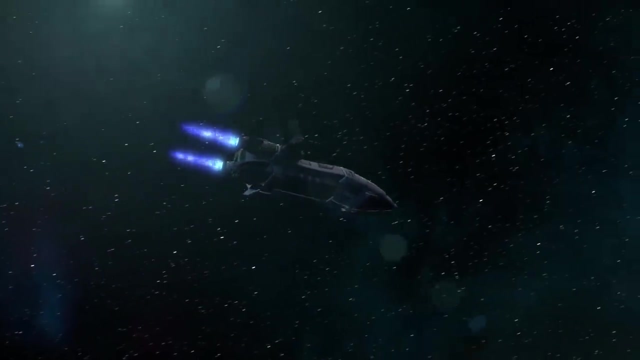 of data without any delay or interference. Another option is to use advanced artificial intelligence that could help spacecraft navigate the vast distances between stars and adjust course as needed, even without any involvement of a human controller. Accurate navigation is key for successful interstellar travel. Even the slightest 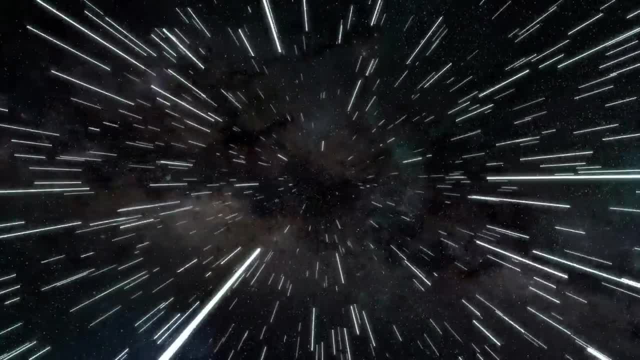 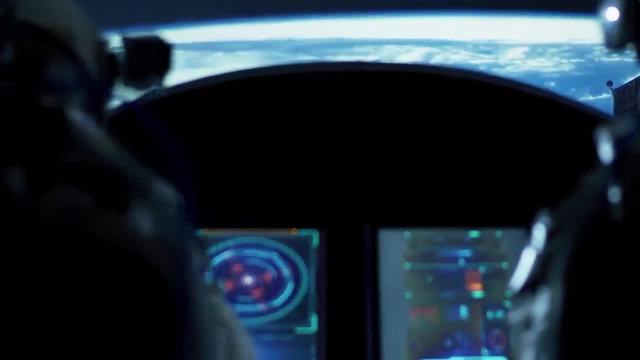 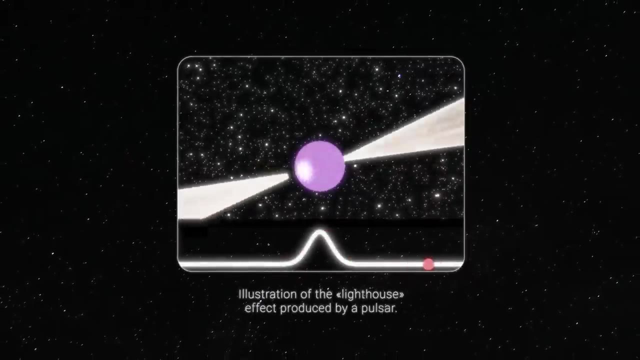 deviation can throw a spacecraft off course for millions of miles. To minimize the risk of this happening, the ships will need incredibly accurate navigation systems, such as ones using pulsars as reference points. Pulsars are highly magnetized rotating neutron stars that emit beams of electromagnetic radiation from their 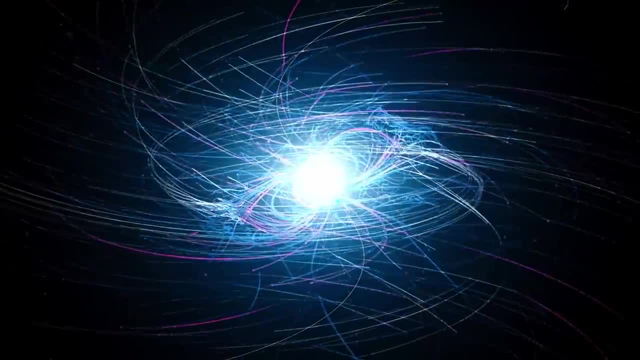 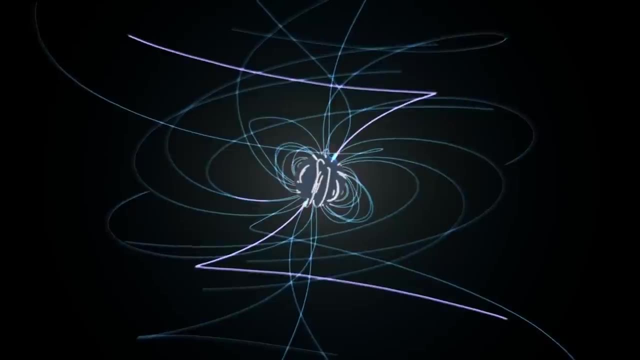 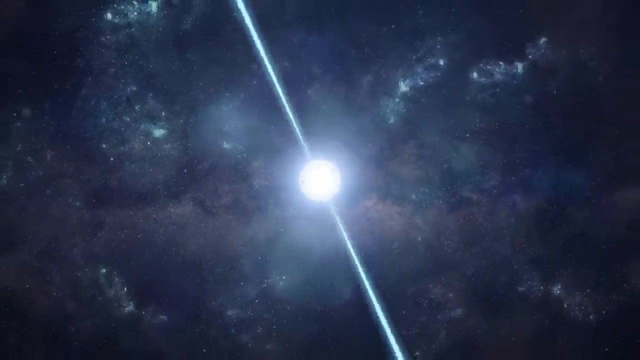 poles. Think of them like cosmic beacons. As the pulsar rotates, it sends out the beam of radiation that shoots through space, creating a so-called momentum. Pulsars are incredibly reliable and predictable, making them ideal candidates for deep space navigation, For example. the technology 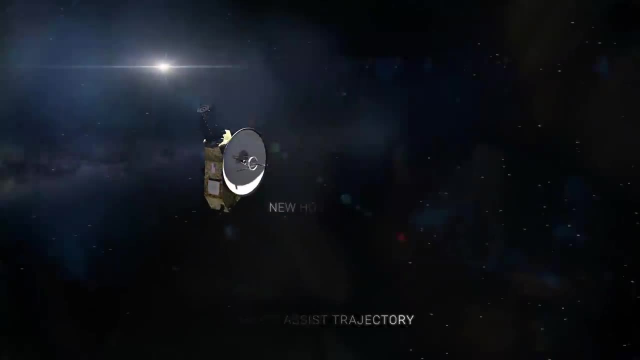 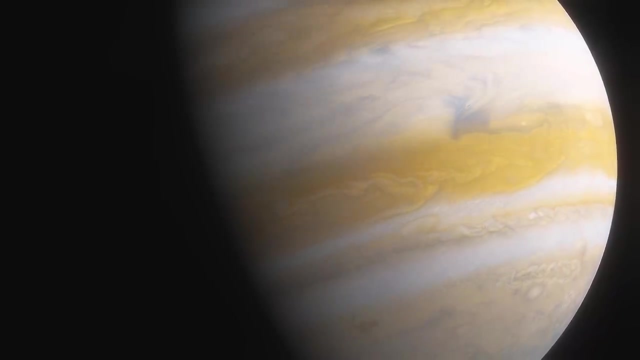 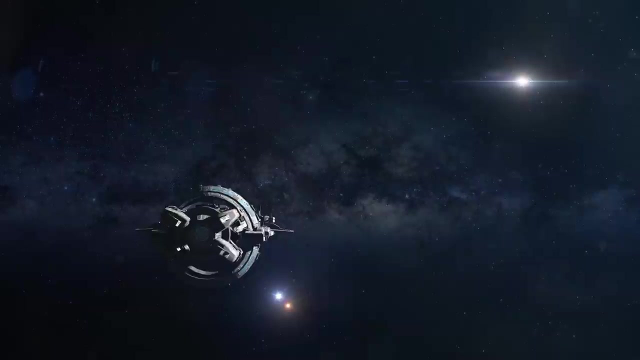 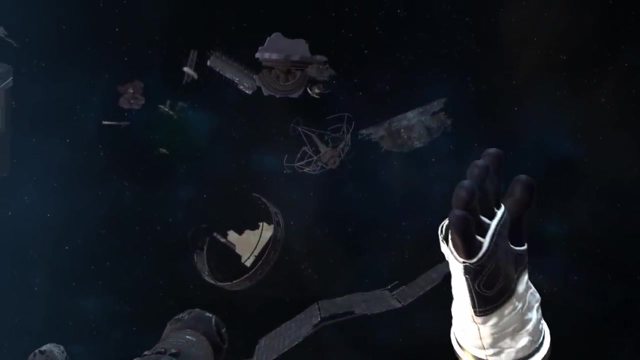 used in the New Horizons spacecraft mission to Pluto relied on Jupiter's gravitational forces to guide the spacecraft to its target. However, as with any complex system, there is always a risk of hardware malfunctioning in some way Without human intervention in real time, these failures can have catastrophic consequences, potentially leading to the loss of 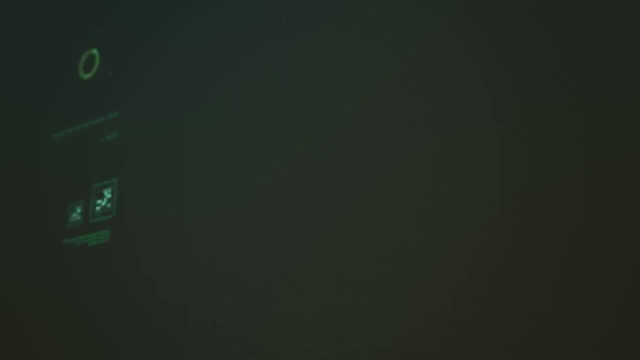 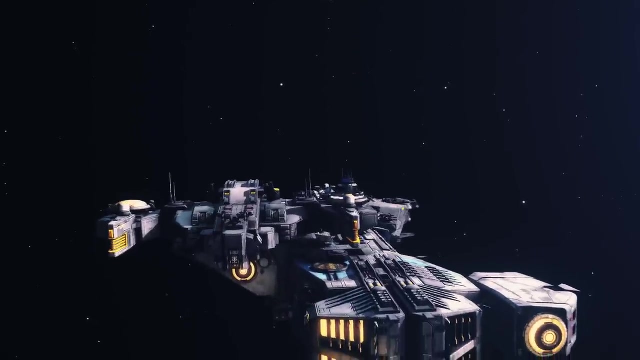 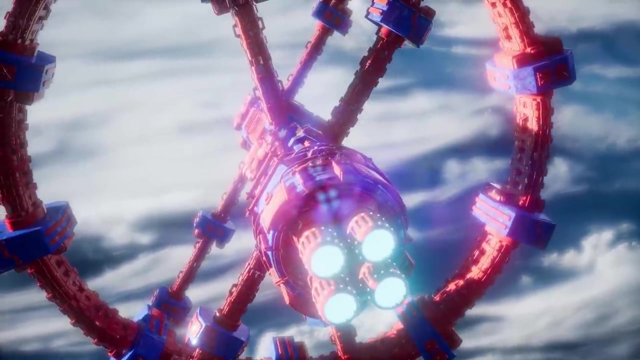 the crew and the mission. This means that the spacecraft will not be able to navigate the space. That is why, in the absence of accurate and reliable communication and navigation systems, a mission to the nearest stars would not have any success, But no matter how highly equipped the ship is as it rushes towards distant stars. 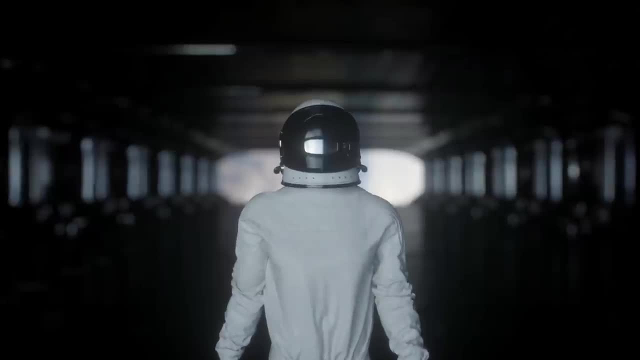 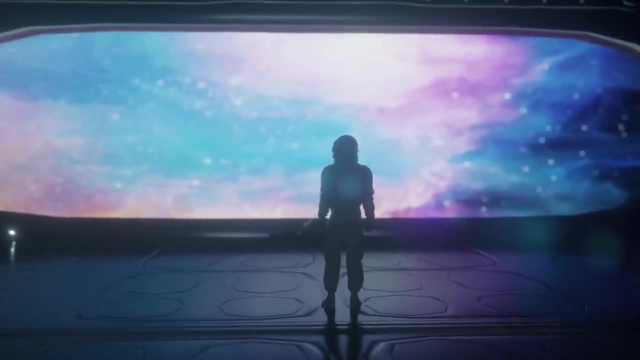 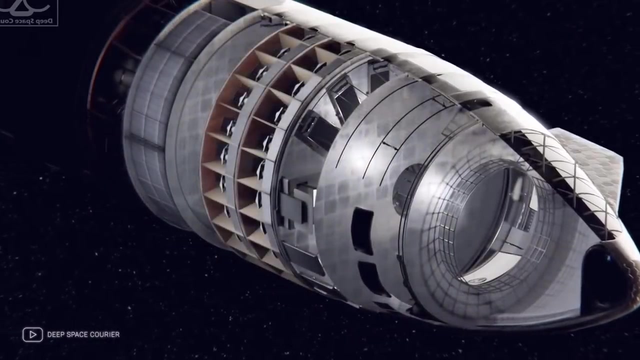 the most important component of the mission are still the people on board. The most important task in interstellar travel is to provide the crew with sufficient resources to survive during the journey. This includes developing life support systems that could provide enough food, water and oxygen. With current technology, it is only possible to 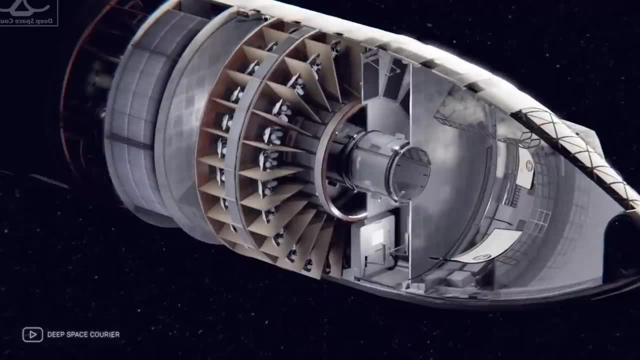 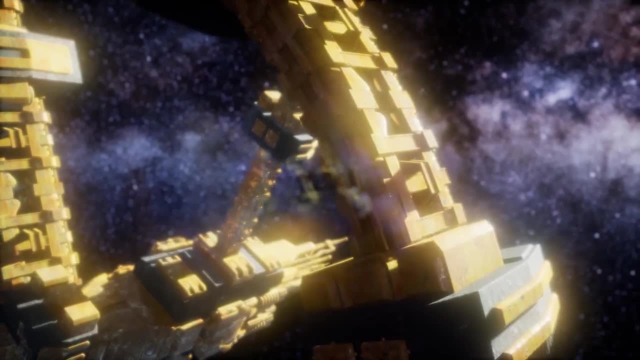 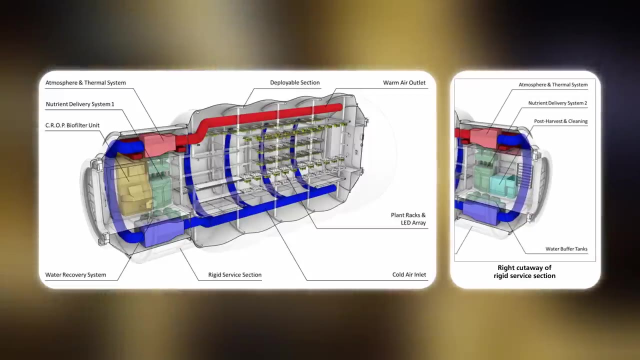 store a limited amount of resources, not enough for truly long journeys. Therefore, we need new technologies and ways to sustain life while traveling over a long distance. One potential solution is to develop regenerative life support systems that can recycle waste and convert it into useful resources. Additionally, the development of advanced 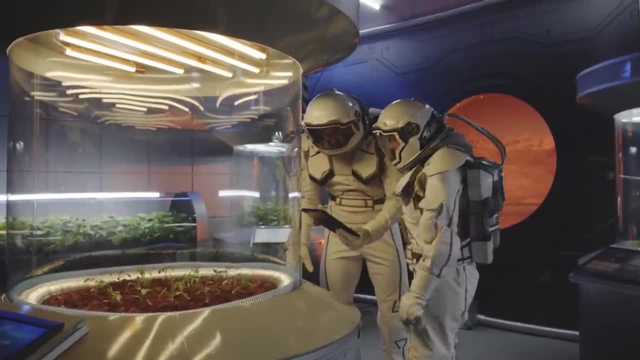 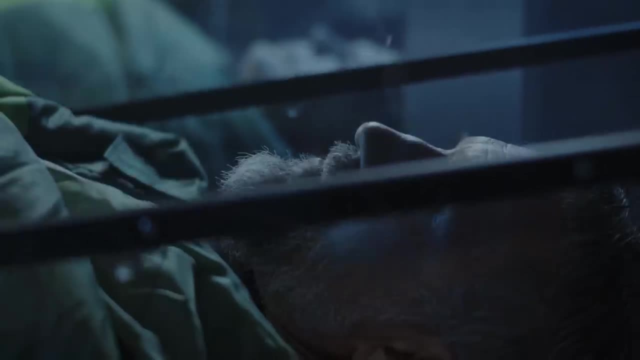 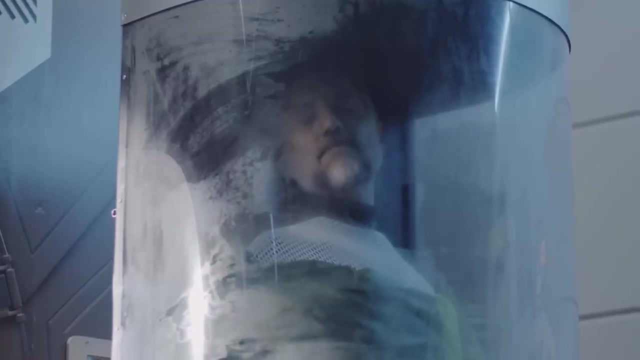 food-growing and oxygen-producing systems aboard spacecraft is a must in research. Another option is to put astronauts into deep sleep for the duration of their journey, similar to the way animals hibernate in winter. Scientists are exploring the use of this technique, known as suspended animation or hibernation, although at the moment it presents significant medical challenges as to how to keep the crew in this suspended state for long periods of time without causing serious health issues, which could significantly reduce the resources and life support systems required. Moreover, prolonged exposure to zero gravity can have detrimental effects on the human body. It leads to muscle atrophy, loss of bone density. 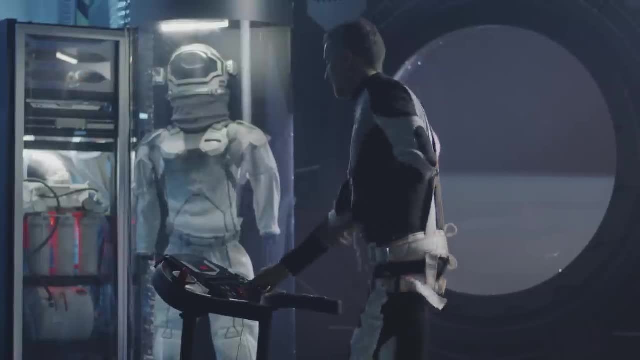 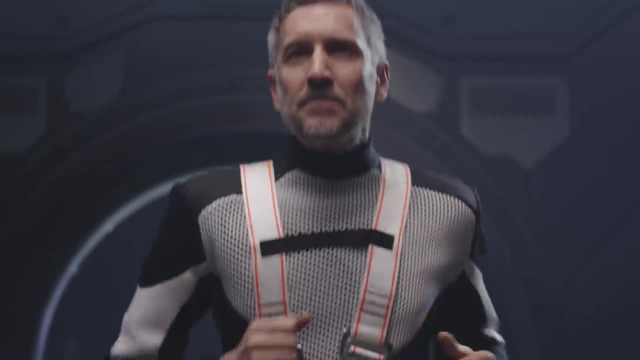 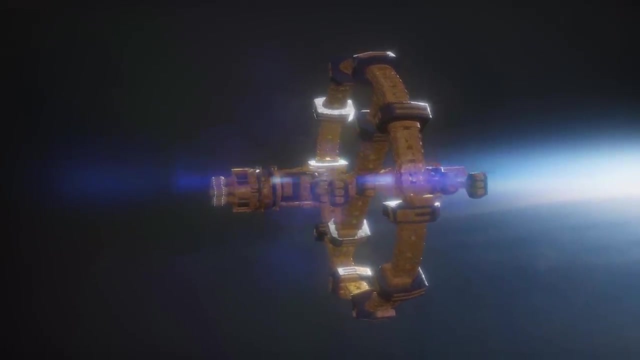 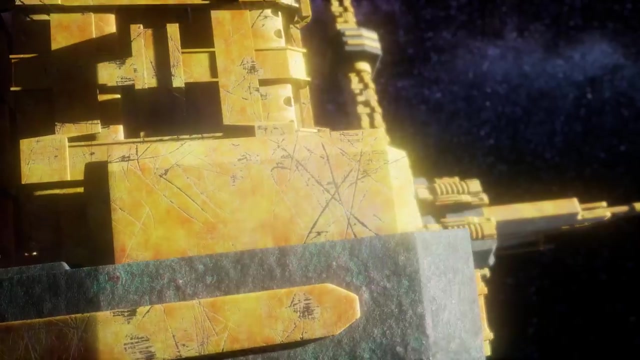 and other physical changes. Therefore, to maintain the health of the crew during the journey, physical exercise and medical intervention may be required. To counteract the negative effects of zero gravity, what may help is an artificial gravity system in place. One way to do that is to maintain the constant rotation of the spacecraft. The 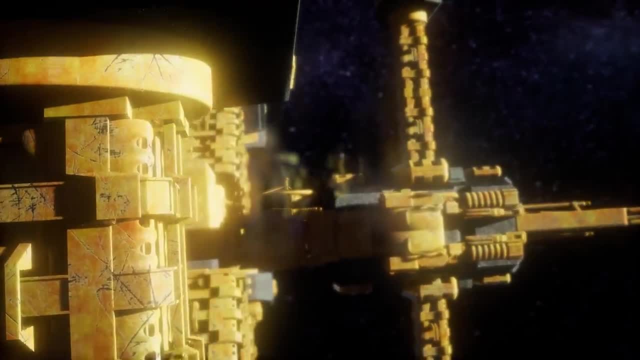 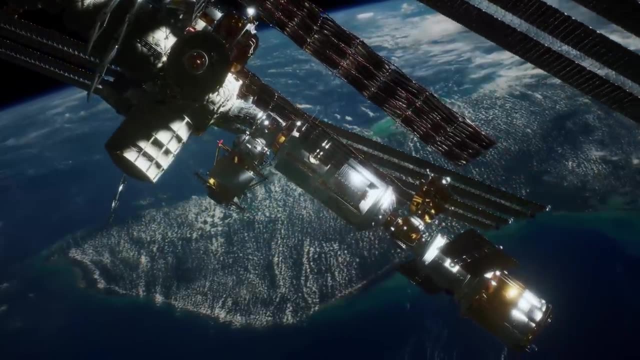 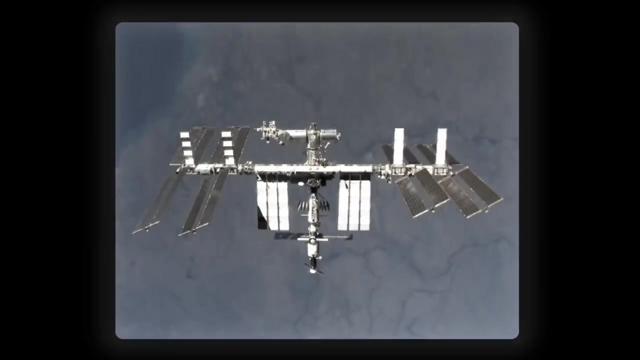 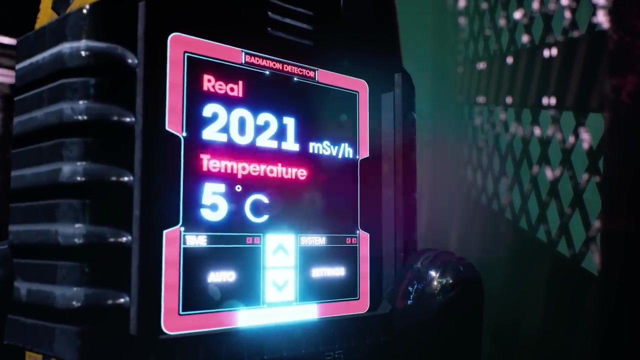 centrifugal force created by rotation can mimic the gravitational force that we experience on Earth. This approach has been researched and successfully tested on various space missions, including Skylab and the International Space Station. Another major health concern when it comes to interstellar travel is radiation. Space is riddled. 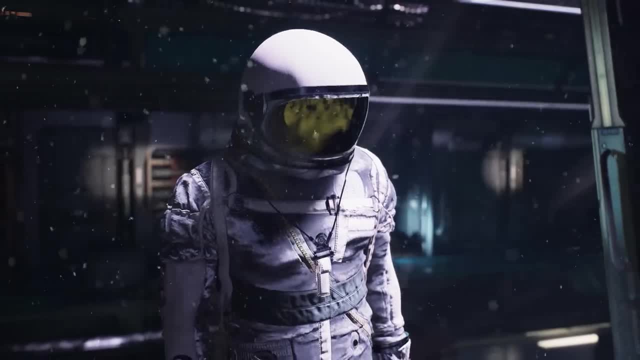 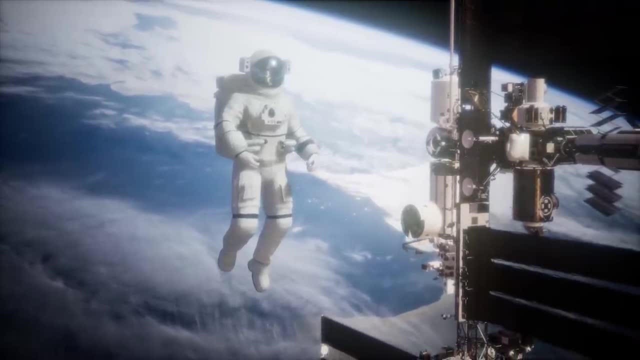 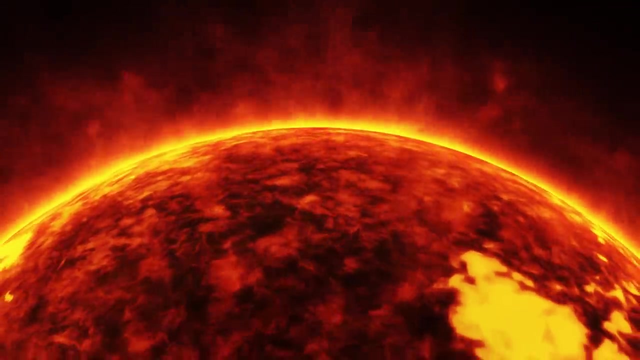 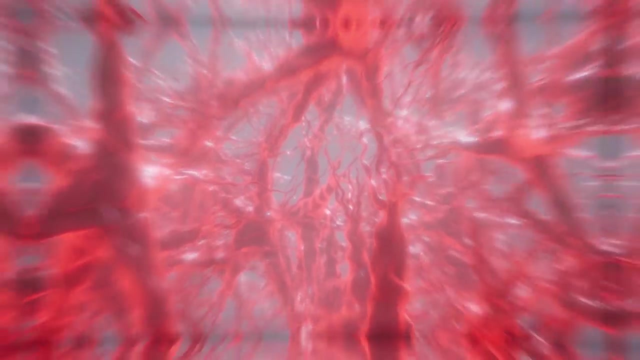 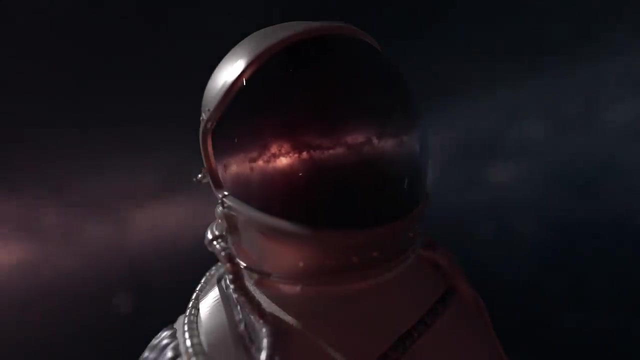 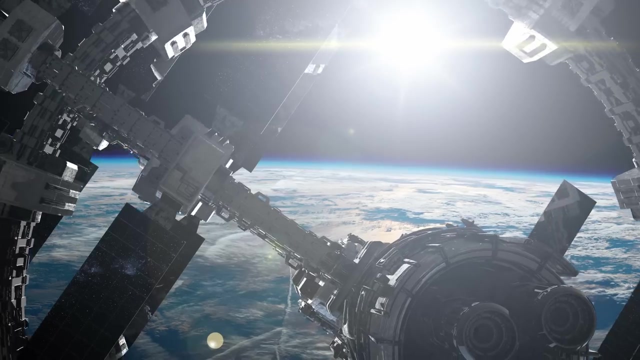 with an endless array of radioactive emissions, long-term exposure to which poses a significant health risk to astronauts. Outside of Earth's protective magnetic field, humans are exposed to high levels of ionizing radiation. Ratings of radiation說 287.3% In a particular room. the OrbIT site shows a total of 0.6 dataset radiation, including cosmic rays and solar flares. Ratings of radiation say that radiation causes damage to human cells, leading to various health problems, including cancer and other illnesses. Additionally, exposure to cosmic radiation can cause genetic damage to DNA that can be passed to future generations. To reduce the risk associated with radiation exposure, the International Space Station must be designed in a way that shields the radar. 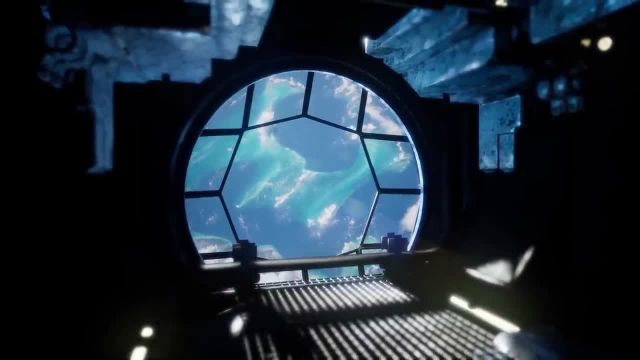 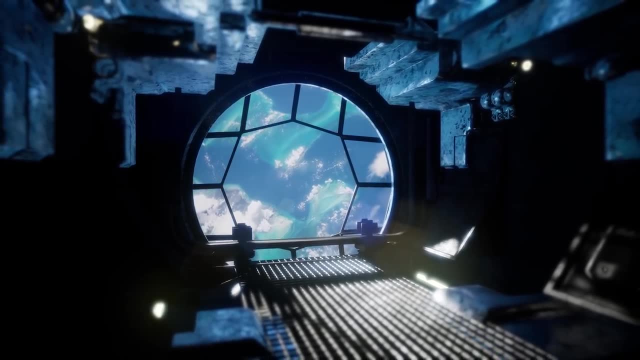 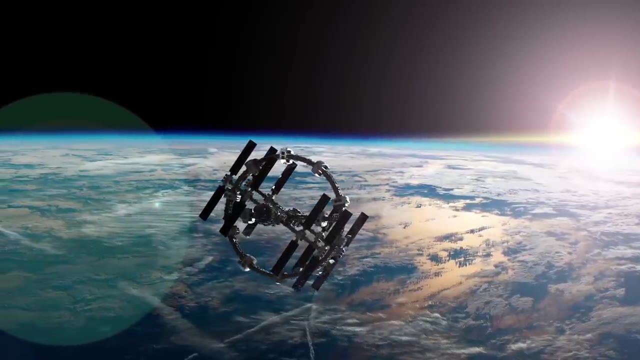 the crew. This shield must be strong enough to block harmful radiation while at the same time being light enough to not significantly increase the weight of the spacecraft. It must be adapted to all types of radiation that the spacecraft may encounter during its journey. To address: 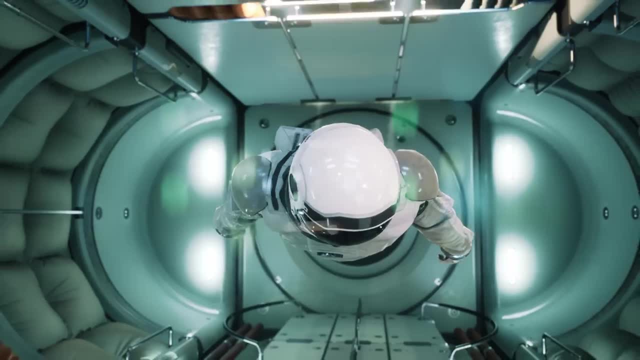 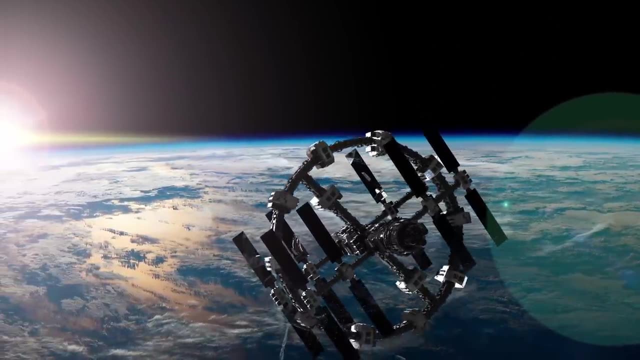 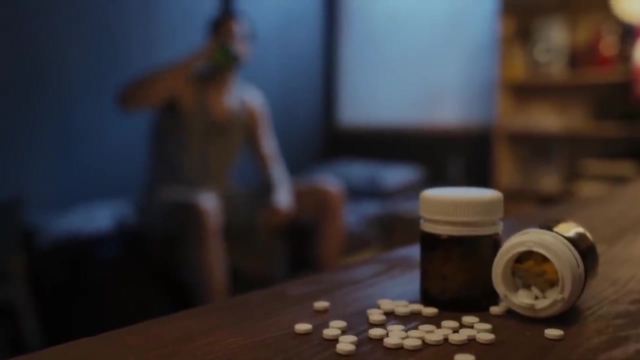 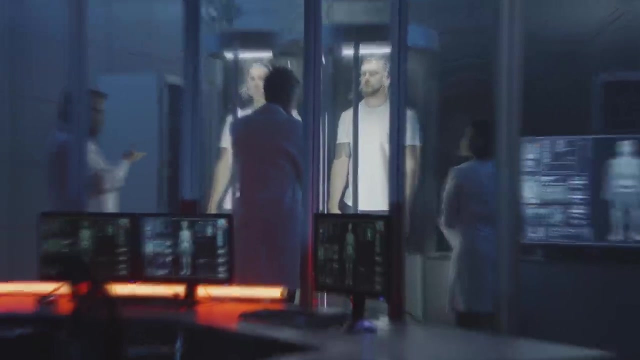 these issues. researchers are exploring various options for protection against radiation, including the use of artificial magnetic fields, as well as advanced technologies and specialty materials. In addition, the crew may need to take special medications or undergo medical procedures to reduce the effects of radiation sickness. In addition to the tiniest radiation, particles. another danger you may encounter during interstellar travel are debris and asteroids that can arrive at the destination and cause a lot of damage. If you are in a situation where you cannot support yourself in the face of the information you are used to, you are likely to get attacked more than your astronaut might. A scenario can be applied to: interstellar travel, presenting us with a dilemma of whether we should launch interstellar ships now or wait for technologies that will generate greater speed and allow new ships to reach destinations faster. The ethical dilemma here is whether it would be fair to the crew of the first. ships to make a senseless sacrifice, in case the rate of technological advancement suddenly started to rise and the crew was dead and the scientific research would not be able to focus on this situation, Whether it would be fair to the crew of the first ships to make a senseless sacrifice. surpass that of the first ships. Put yourself in the shoes of a pioneering crew member in another star system. You've spent decades or even centuries in space wondering if newer and faster ships may have arrived at your destination long before you. This dilemma raises deep questions about the value of human life, the responsibility for space exploration. and the importance of progress. Waiting for new technologies could lead to faster, more efficient travel, But it could also mean that the first crew would suffer or be exposed to dangers that future generations may not even have to face. Conversely, launching ships now can be seen as unfair to the crew, as they will not benefit from the same advanced technology. that future generations will. Ultimately, the final decision will depend on how society perceives the importance of progress in research in relation to the value of human life. In a quest to understand the vast and mysterious universe, science has long mastered the powerful tool of logic. But even when using it, it's not always easy. The most rigorous methods and the most advanced technologies, paradoxes inevitably arise—contradictions that challenge our understanding of the world. One such paradox is the dark sky at night. How is it possible that we're surrounded? by an infinite number of shining stars, and yet the sky remains dark. The other is the nature of dark matter in the observable universe. It has negative pressure and acts as a repulsive force, counteracting the gravitational force of matter and causing the universe to expand at an accelerated rate. This acceleration would help to flatten the Universe. Another solution is the concept of inflation. According to the theory of inflation, the universe underwent a rapid expansion in the early stages of its formation. as space expands, the geometry of space changes. The universe becomes a barrier to all relativism, and so becomes flatter. To help you understand, imagine a balloon. as it fills with air and inflates, Its surface becomes smoother and flatter. This type of expansion would smooth out any initial density changes, making the universe nearly flat. The third solution is the multiverse theory. which suggests that our universe is just one of many. According to this theory, there are a large number of universes. Based on this, the likelihood that one of them will be flat is much higher than if there was only one universe. The monopole paradox is yet another example of an unyielding mystery of the universe. This is a paradox that comes from the observation that there are no observable magnetic monopoles, despite the fact that their existence is predicted by several things. The monopole paradox is a paradox that comes from the observation that there are no observable magnetic monopoles, despite the fact that their existence is predicted by several things. The monopole paradox is a paradox that comes from the observation that there are no observable magnetic monopoles, despite the fact that there are no observable. magnetic monopoles, despite the fact that there are no observable magnetic monopoles. Magnetic monopoles are hypothetical particles with a single magnetic pole, while all known magnets have a North and a South pole. The existence of these hypothetical particles has been predicted in theories such as the grand unified theory. a grand unified theory or GUT and quantum gravity theories. However, despite great efforts and extensive research, no magnetic monopoles have been found. Nonetheless, despite their elusive nature, there are many theories attempting to explain their apparent absence. One possible explanation for the absence of magnetic monopoles is their inspection of the black hole information paradox, or Hawking's paradox, as a problem in theoretical physics. Scientists suggest that black holes absorb information, thereby irretrievably destroying it. But what do we mean by information? Information in the context of this paradox refers to quantum parameters that describe: 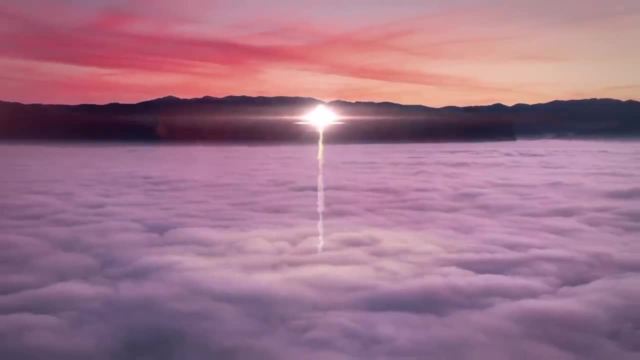 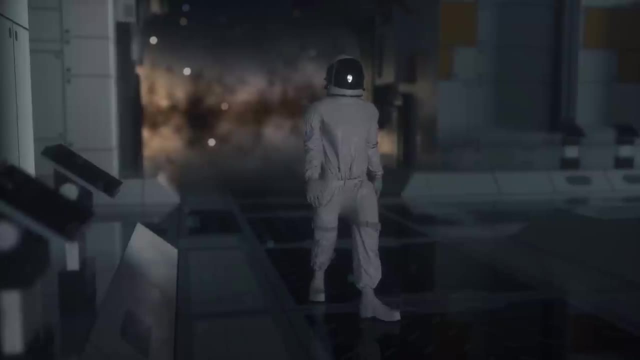 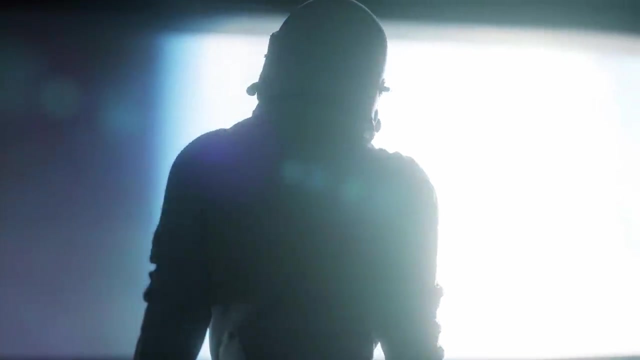 the state of a physical system. These parameters contain all the information needed to fully define the state of the system. They play a central role in the principles of quantum mechanics. Quantum mechanics believes that: • The entirety of information in the universe is neither limited nor destroyed. 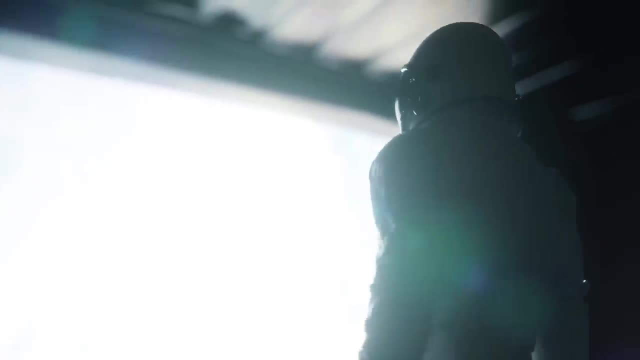 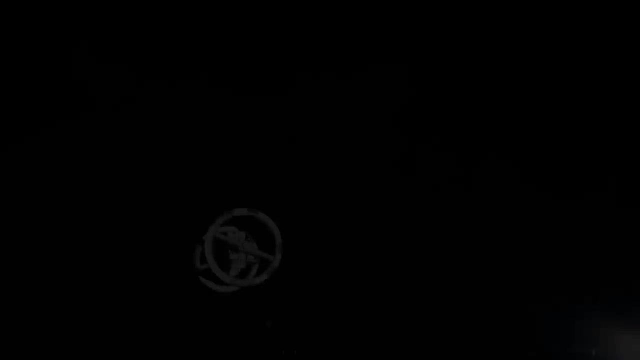 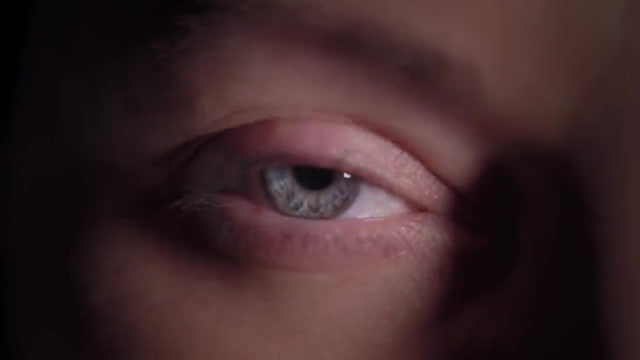 Now let's go back to how this paradox arises. It happens because of the contradiction between the two most established theories in physics – quantum mechanics and the general theory of relativity. Up to a certain point, the laws remain intact and have no effect on each other. 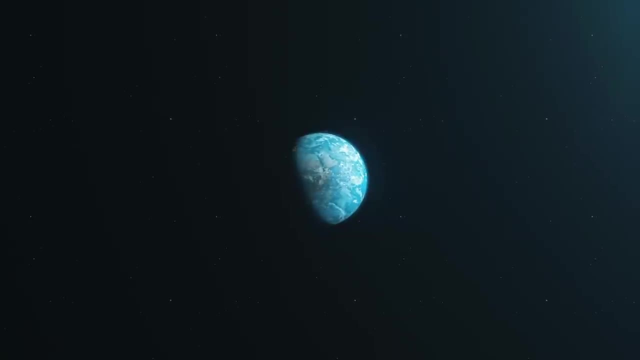 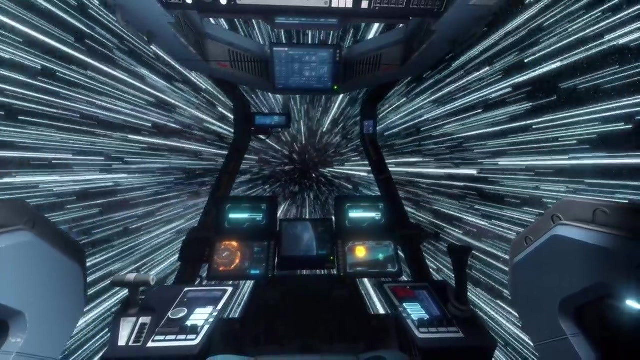 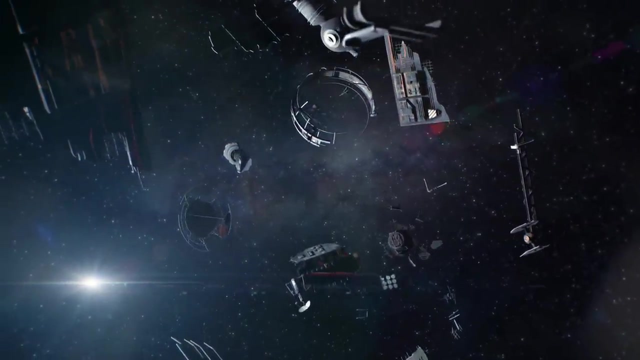 But this only happens before the Hawking radiation comes into play. 2. Information Paradox. The information paradox was first brought to the forefront of scientific discourse by Stephen Hawking in the 1970s. He proposed that black holes emit thermal radiation that lacks any information about. 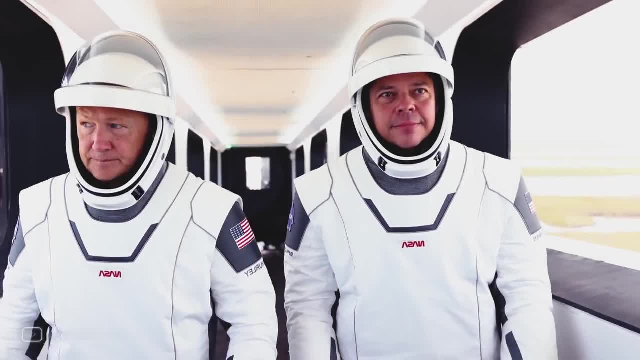 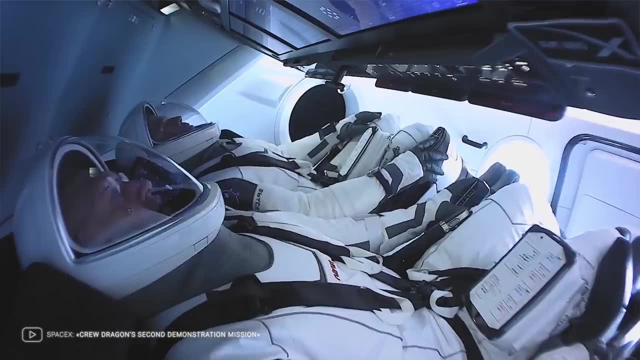 the matter that has entered the black hole. This led to the idea that information is forever lost when it enters a black hole And the fundamental laws of physics are not deterministic. The information paradox has been the subject of much discussion. The information paradox has been the subject of much discussion. 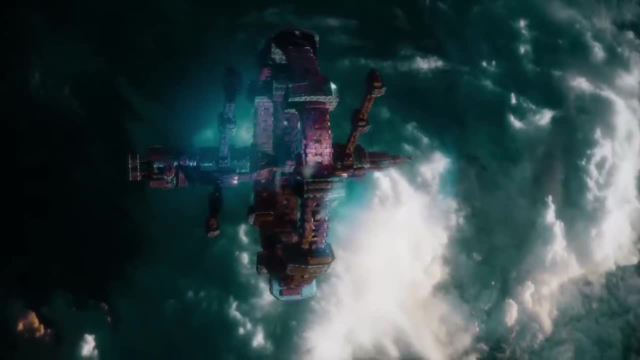 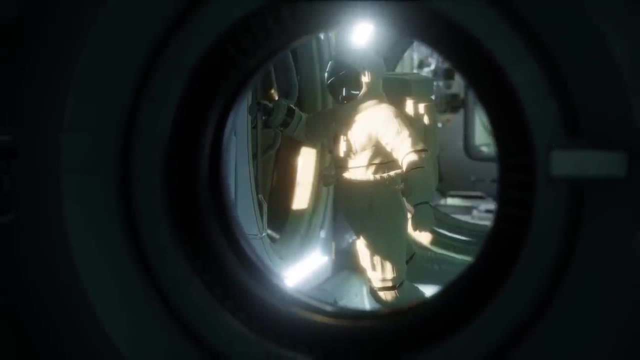 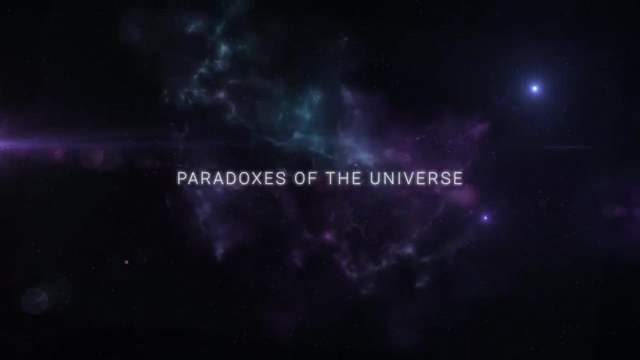 The information paradox has been the subject of much discussion, An idea that suggests that the information sucked into a black hole has been spread. On one side of the horizon, the laws of general relativity operate. On the other, the laws of quantum mechanics operate. 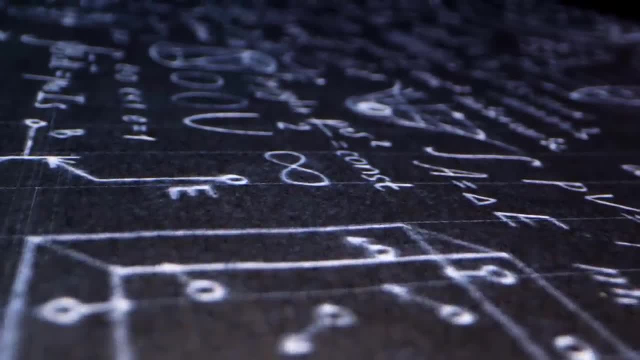 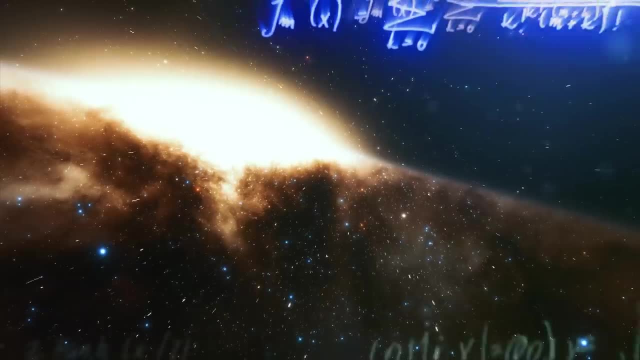 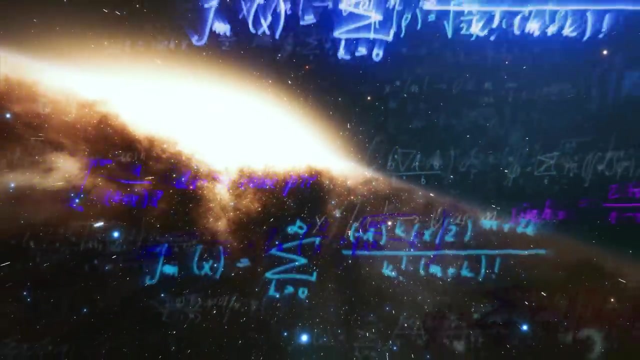 Information falling into a black hole is encoded on the horizon in a way that is consistent with both sets of laws. 2. providing a possible solution to the information paradox. Another proposed solution is the firewall paradox, which states that information is not lost, but instead stored by a firewall of high-energy particles surrounding the black. hole. Despite all the aforementioned theories, the information paradox remains one of the most difficult and important unsolved mysteries in theoretical physics. It is integral for our understanding of the nature of black holes, the principles of quantum mechanics and general relativity and, most importantly, the ultimate fate of the universe. Dark Matter and Dark Energy Paradox. The dark matter-dark energy paradox, also known as Bentley's paradox, is a problem in physics that arises from a discrepancy between the observed behavior of the dark matter and the dark energy paradox. What is the standard model of the universe? A key piece of evidence for the existence of dark matter and dark energy is the observed gravitational effects of these mysterious substances. The standard model of cosmology based on general relativity predicts that the observed gravitational effects of the rotation curves relationships with galaxies and the large-scale structures. of galaxies, clusters and the operating slow- transient manner of interaction are %. clusters must be much weaker than they actually are. The discrepancy is known as the gravitational paradox, and it has led scientists to suggest the existence of dark matter and dark energy to compensate for those gravitational effects. Dark matter is estimated to make up about 27% of the universe and it is speculated to exist based on its gravitational effect on visible matter. It doesn't interact with light or other forms of electromagnetic radiation, which makes it difficult to detect directly. Scientists have proposed various candidates for the role of dark matter, including WIMPs, weakly interacting massive particles and axions. However, despite decades of research, neither of them have been detected with any degree of certainty. Scientists also believe that dark energy makes up about 68% of the observable universe and is responsible for the acceleration of the expansion of the universe. Its existence is confirmed based on observations, but the nature of dark energy is not entirely clear. The most popular explanation for dark energy is the cosmological constant proposed by Einstein, which is a form of energy evenly distributed throughout the universe. However, this explanation raises some issues, such as the cosmological constant problem and the coincidence problem. These problems stem from the fact that the observed value of the cosmological constant is much lower than the theoretical predictions, as well as the fact that it has the same order. of magnitude as the density of dark matter. It's also worth mentioning that the current standard model of cosmology, the lambda-CDM model, which uses the concept of dark matter and dark energy, is not the same. It's also worth mentioning that the current standard model of cosmology, the lambda-CDM- which uses the concept of dark matter and dark energy in carbonerte, corresponds with a wide range of observational data and is considered the most successful model of the universe to date. Bentley's Paradox refers to the fact that, even though dark matter and dark energy make